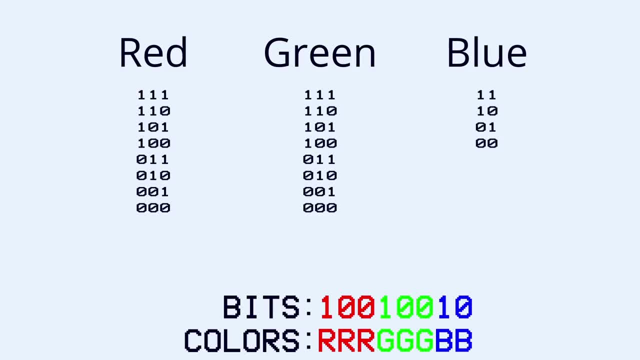 why most systems and applications used one less bit for the blue colors. Using this, we can define 8 shades of red, 8 shades of green and 4 shades of blue, And all combinations between them, Giving developers a total of 256 different colors to work with. 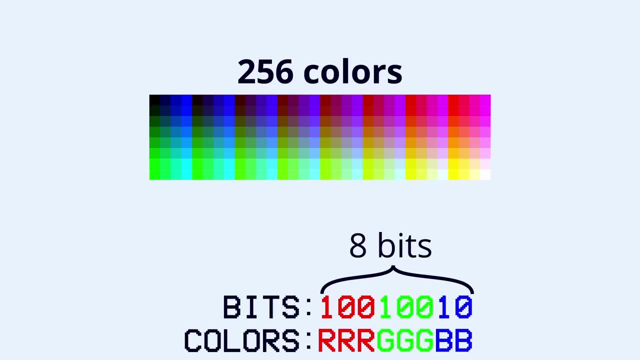 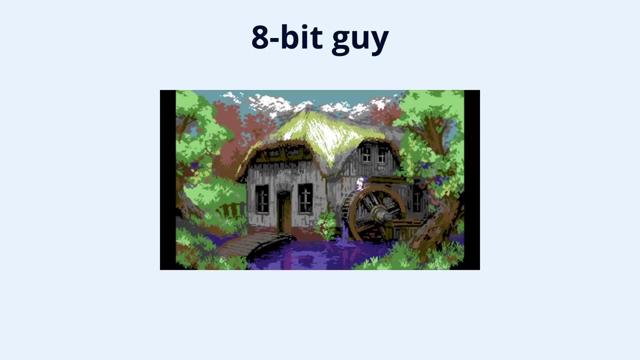 This is the nostalgic 8-bit art style you know from early Nintendo games. Sometimes, for games with a lot of blue shades, developers chose to use more bits for the blue data, Trading it off for less green or red shades. If you want to know more about how exactly old school graphics worked and what clever 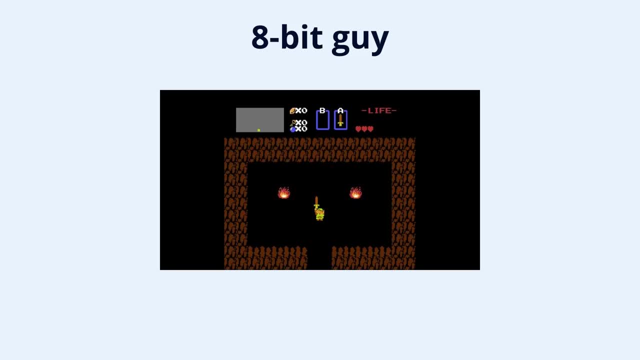 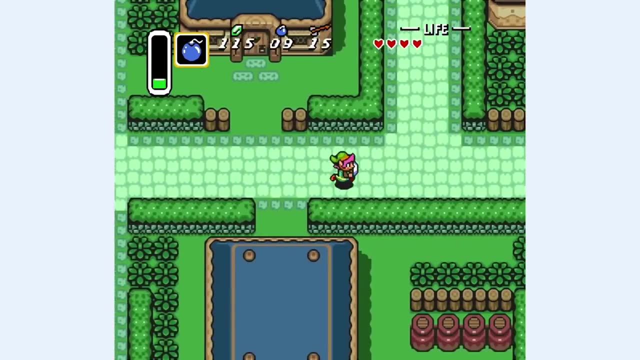 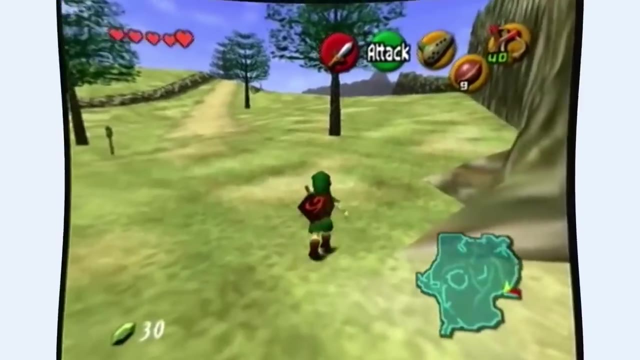 tricks engineers used to work around their limitations. Check out this explanation from the 8 bit guy. Skip forward a few years. we've gone from 8-bit to 16-bit games. Computers could hold more data, which caused graphics to improve, And as computers became more powerful, 3D games became. 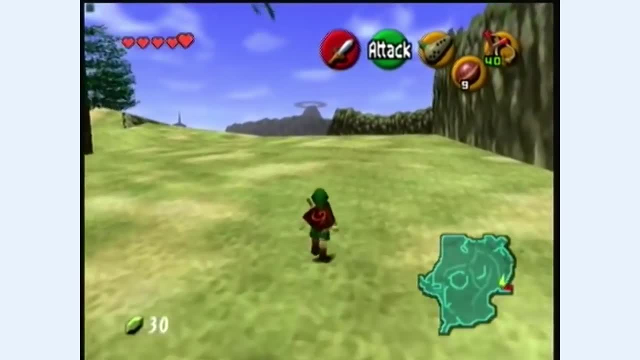 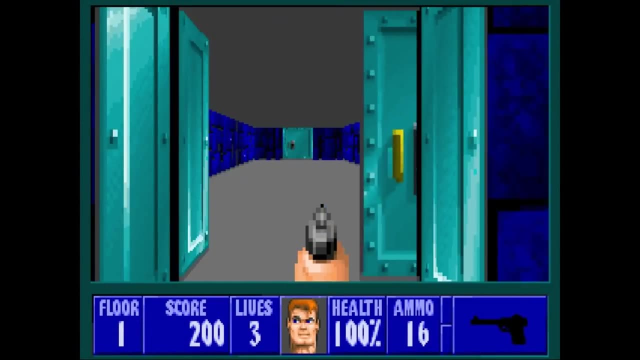 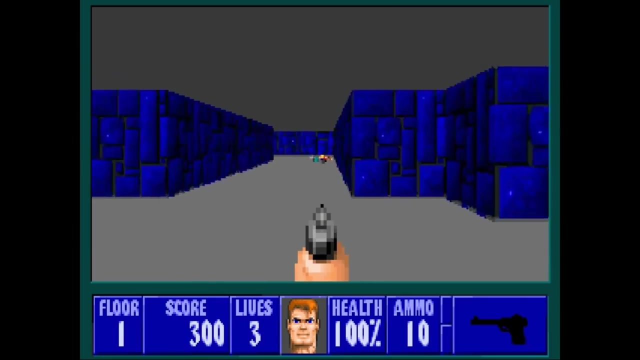 more and more common, And when I am talking about early 3D games, one example immediately comes to mind: Wolfenstein 3D. However, at the time, video cards didn't really have support for rendering 3D graphics yet. So, knowing that, How did Wolfenstein create a 3D environment To fake the 3D effect? it? 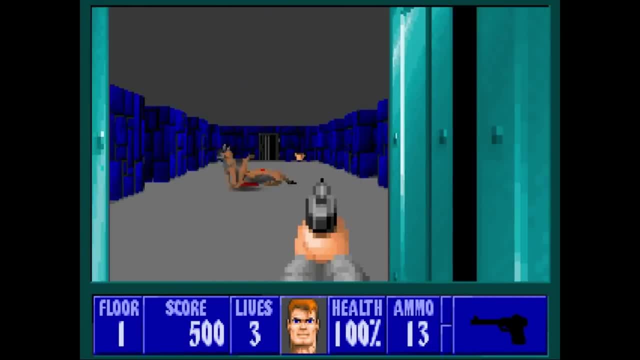 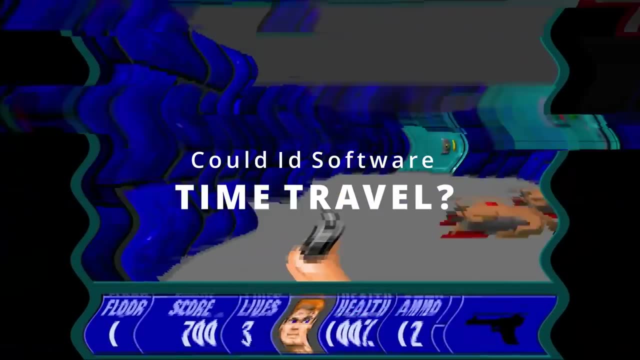 used ray tracing. 3D communication doesn't always happen in great quality, So to test 3D Draw 없이 a minute, That's what that used video card used today. Was Wolfenstein that far ahead of its time? Did its software possess the power to time travel? Well, no. 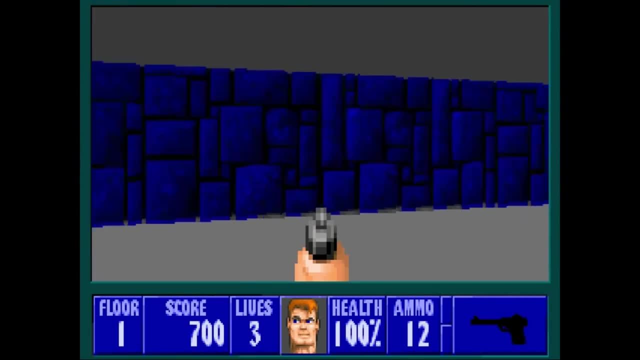 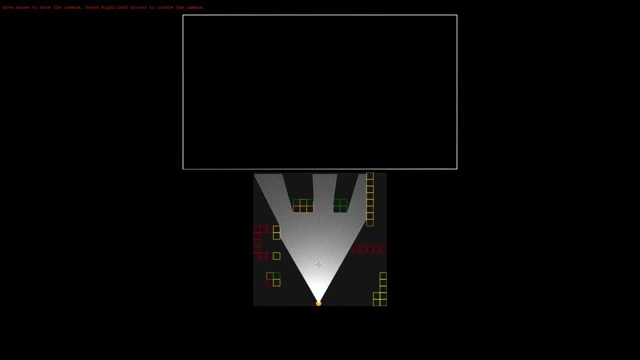 You see, the ray tracing used in Wolfenstein was actually much simpler because it used 2d ray tracing. The way it worked was kind of like a top-down shooter. It used a 2d map for the environment and for every frame it traced where the walls were, with rays shooting from the players position, The 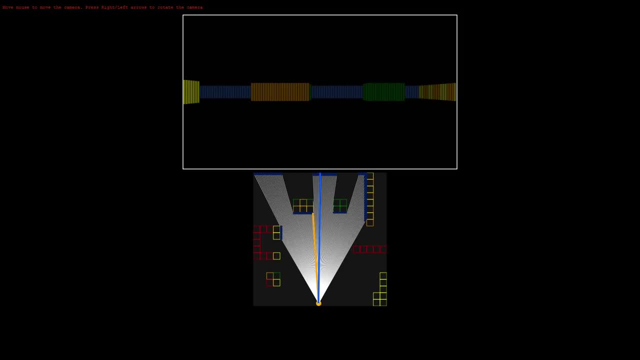 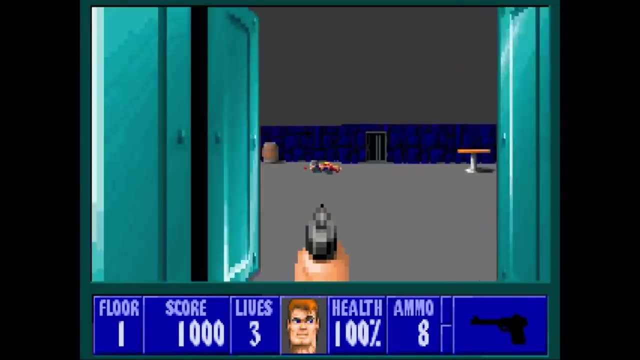 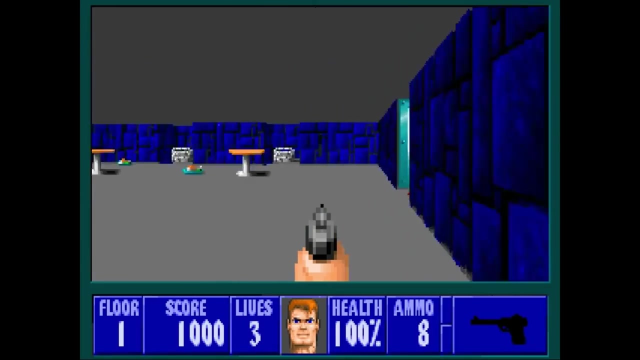 length of those rays determined how far away a wall was and thus how high the wall should be drawn. It was actually a pretty common technique at the time in game engines for faking 3d environments, Commonly referred to as ray casting. This made for some pretty convincing 3d effects on hardware that didn't even 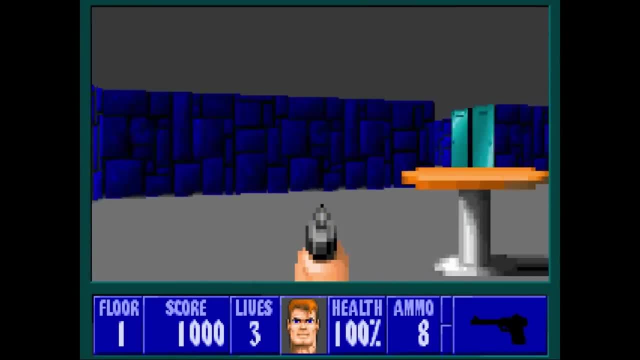 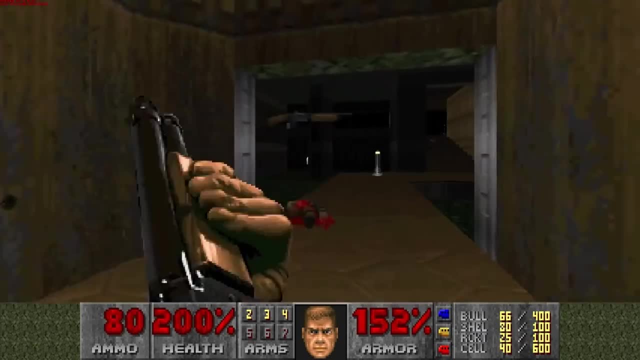 support 3d environments. Game developers can be so clever. The next iteration of 3d rendering was Doom. As you can see, Doom allowed for much more complex rendering than Wolfenstein. There are stairs, elevated rooms, enemies above and below you, All of which was 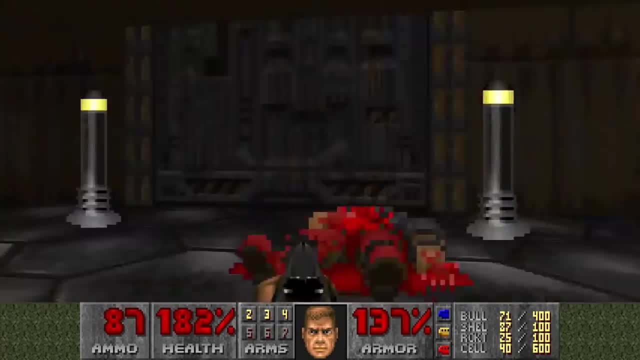 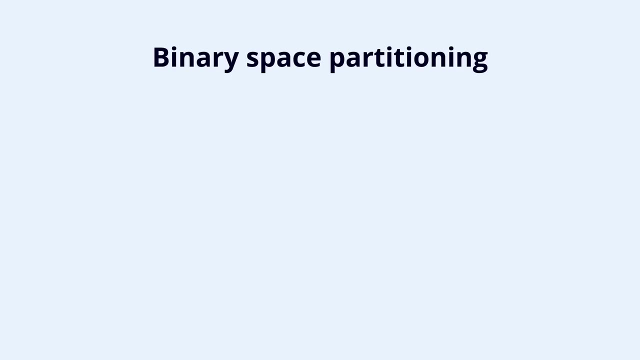 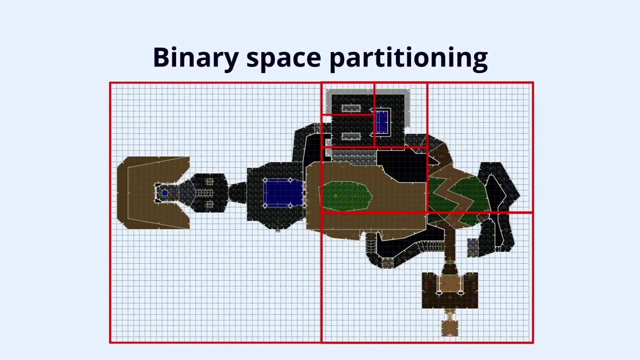 impossible in Wolfenstein. So what did Doom do to allow these more complex environments? Well, it used a technique called binary space partitioning. This technique starts with slicing the world into manageable pieces. Basically, we keep slicing the remaining space in half until we have slices of the environment. 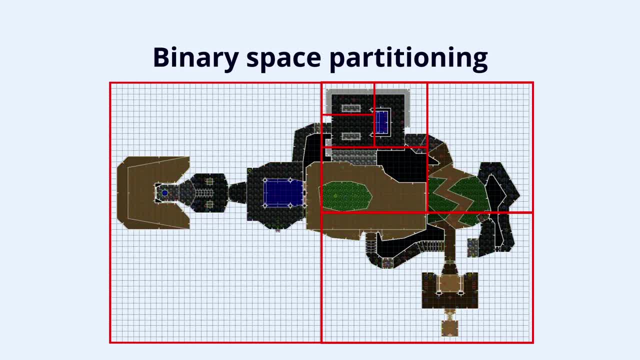 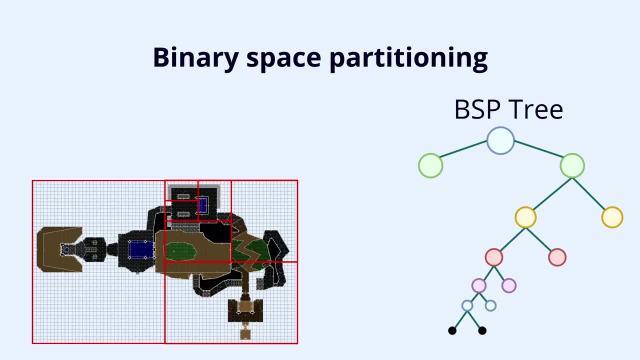 which are small enough for our computer to handle. All of this information is stored in the data tree. Once this preparation is done, we can render our world. To do this, we check what node our player is in and then render the nodes around him. This is where our data tree comes in, Because our tree goes from. 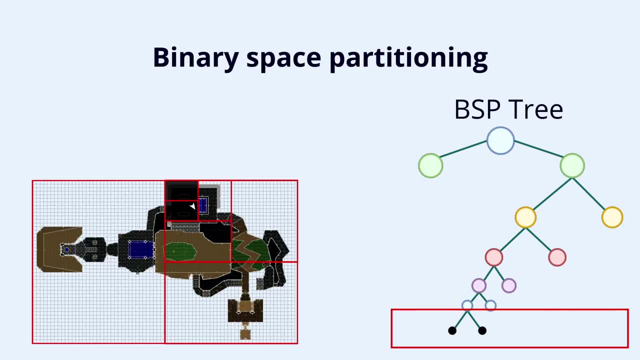 larger to smaller spaces. we can quickly find what part of the world our player is in by repeatedly asking the question which one of these nodes contains our player? So we start at the top, then we ask which one of these nodes contains our player And we find our player is in the right node. 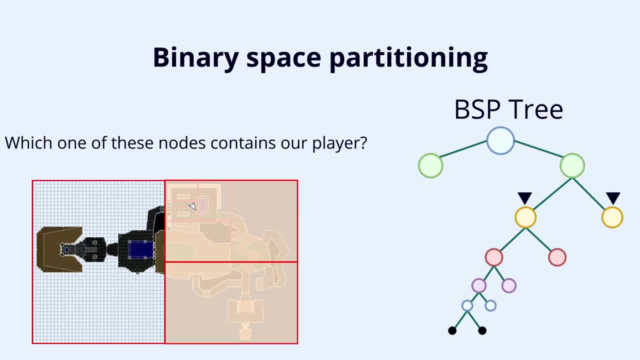 Then we go one level deeper and ask the same question. This time the player is in the left node. We continue on until we reach the very bottom of our tree and we know exactly where our player is in the world. With this information we can start. 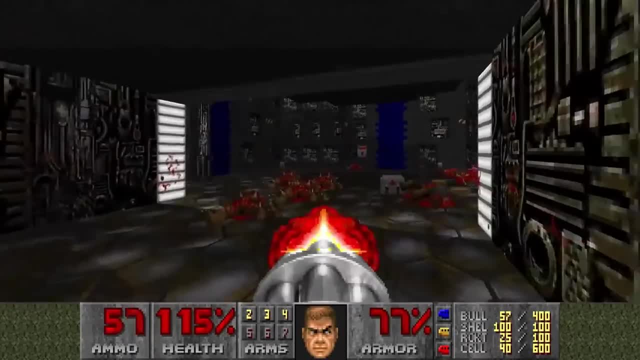 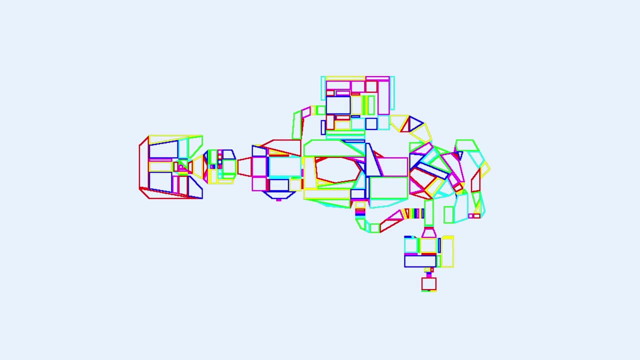 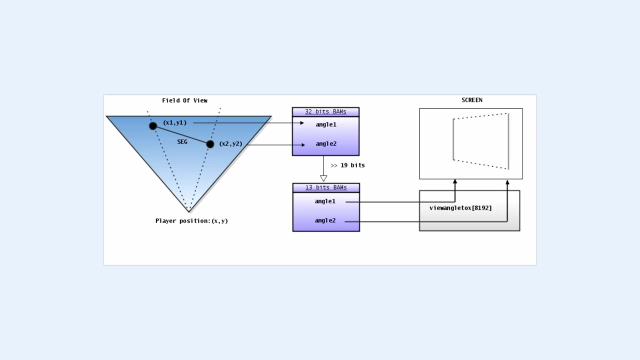 rendering our room. The way Doom renders his walls is different from the ray casting technique we've seen before. As we've just seen this time, the world is divided into many small segments. When rendering, the engine then determines the segment by measuring the walls: distance from the players, perspective lines, Doing. 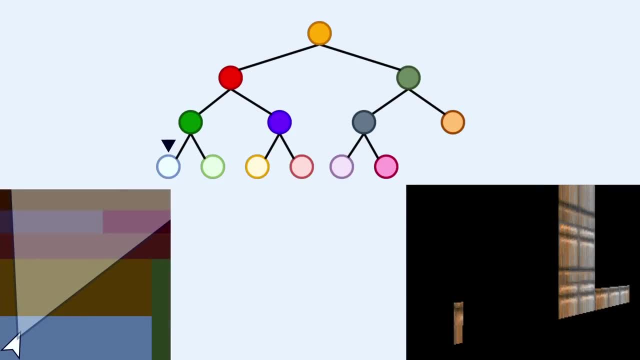 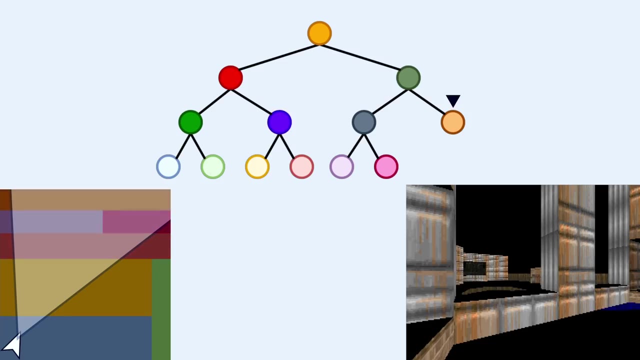 this. each wall in the segment can determine what angle it needs to be drawn at to appear in the correct perspective. We draw all the walls from the closest segment first, Then we have up one node and render the next closest segment, Then again and again until our screen is completely filled. Then the 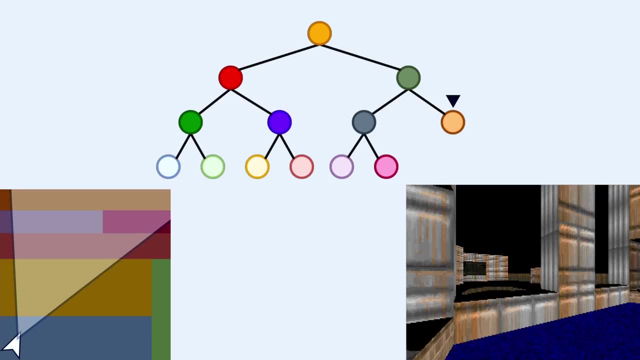 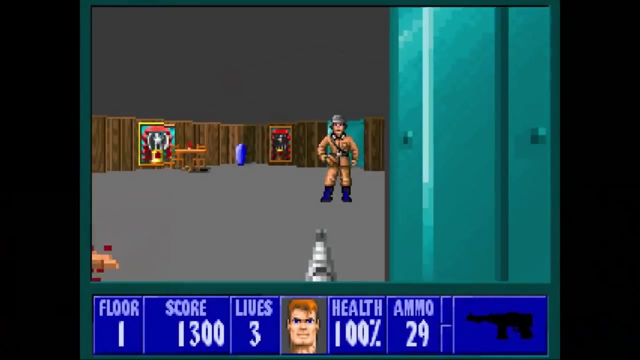 floors and ceilings are drawn and finally the game sprites. Once there are no pixels left to fill, we can stop and our render is complete. Notice how we draw the rooms from near to far. This ensures that we don't draw any obscured areas, saving us a lot of computation power. By rendering our world this way, we are no. 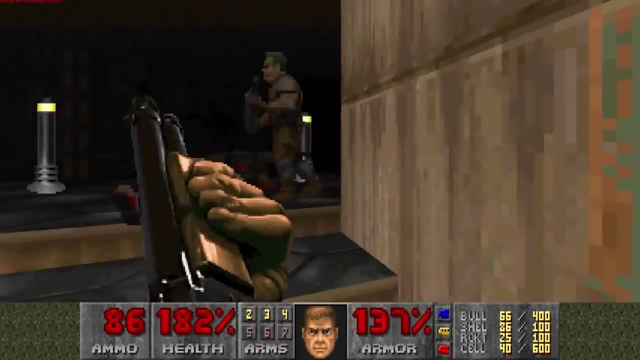 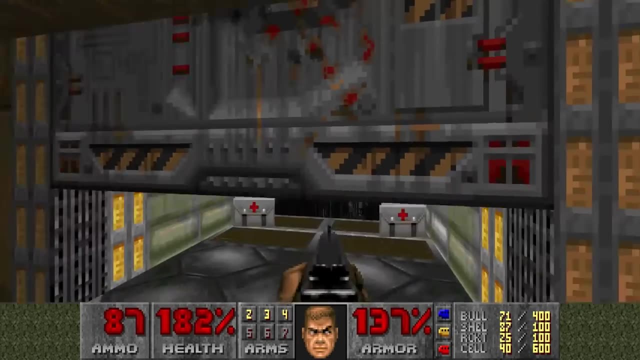 longer bound to the flat 2d environment we saw in Wolfenstein, Because we don't really care what our worlds look like. We can have things like stairs, platforms and elevated rooms, and all of that without using any 3d rendering hardware. But then 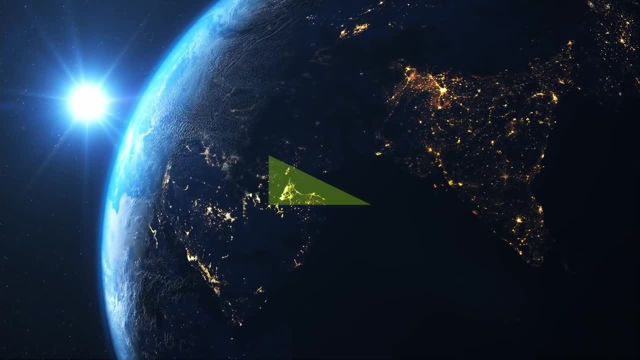 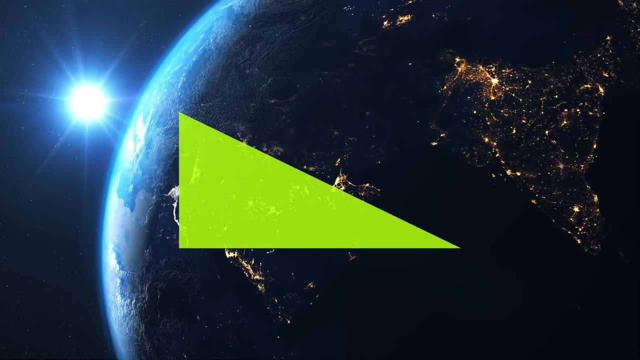 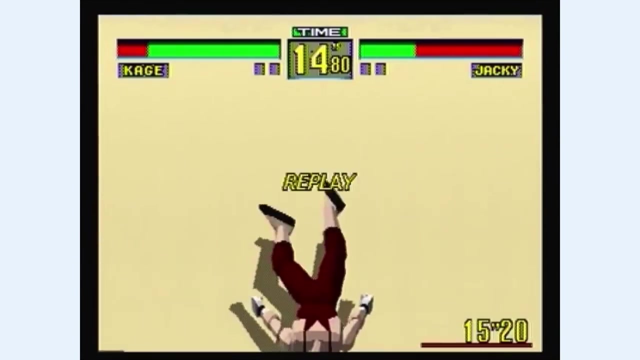 something came that changed the gaming world forever, Something that made the impossible possible and that could make all your virtual dreams come true, Something that could render Triangles Lots and lots of triangles. I'm talking, of course, about the first 3d graphics cards. For the first time, it was possible to 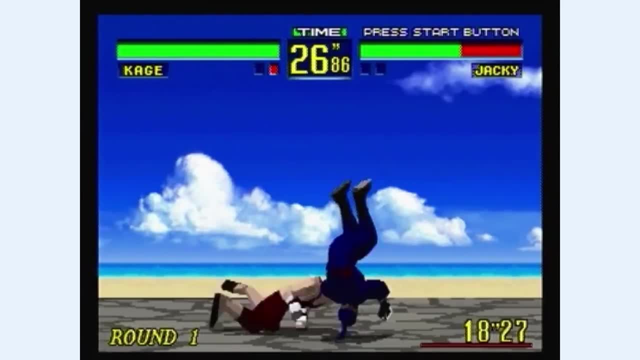 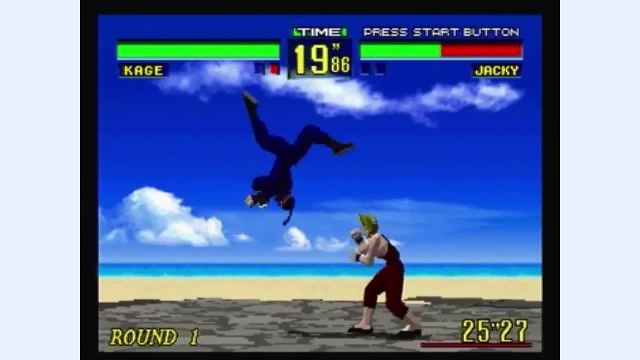 display true 3d graphics and, surprisingly, the way 3d rendering was done back then is pretty similar to the 3d graphics cards we saw in Wolfenstein, Similar to what we use today. As I said before, 3d graphics work by using. 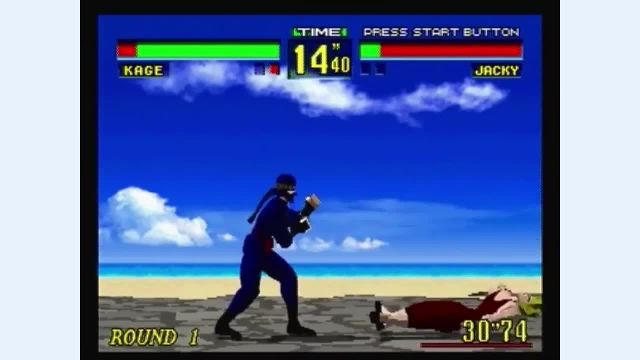 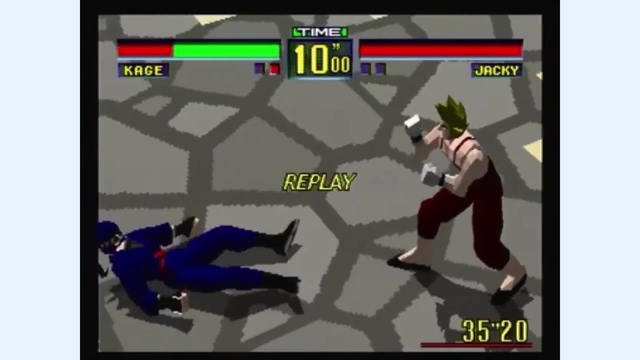 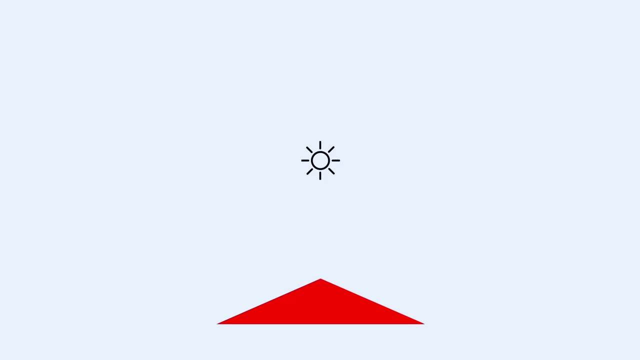 triangles. Everything you see in 3d graphics is secretly just a bunch of triangles coupled together to form complex 3d models. But how do these coupled together triangles produce realistic graphics? The basic principle is that for each individual triangle, you can calculate how bright it should be based on its angle towards a light source. The 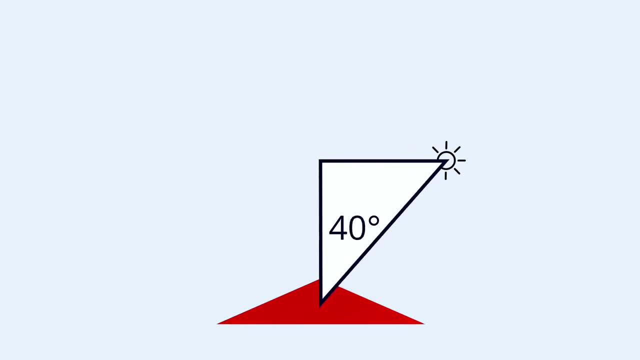 more directly it faces the light, the brighter it will be. Putting all of this together and having each triangle change its brightness based on its angle towards a light gives 3d models their sense of depth. This is called shading In its simplest form. you would change the brightness of the entire surface of the 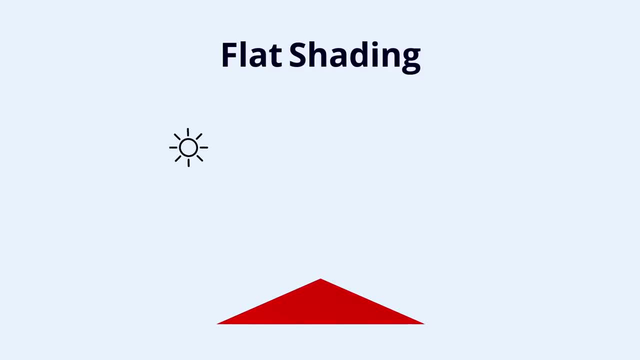 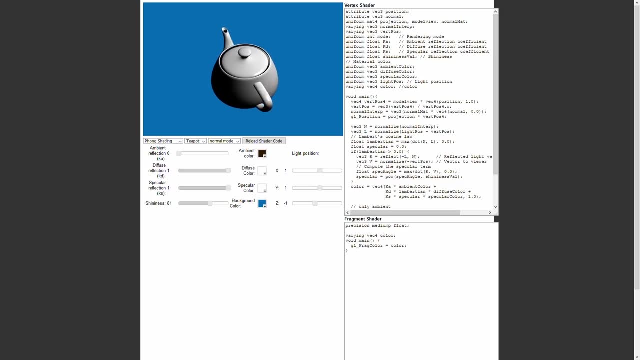 triangle based on its angle towards a light. This is called flat shading and can be seen in very early 3d games. But we can also perform more complex calculators on our triangles, Where all the pixels inside the triangles are interpolated in such a way that our 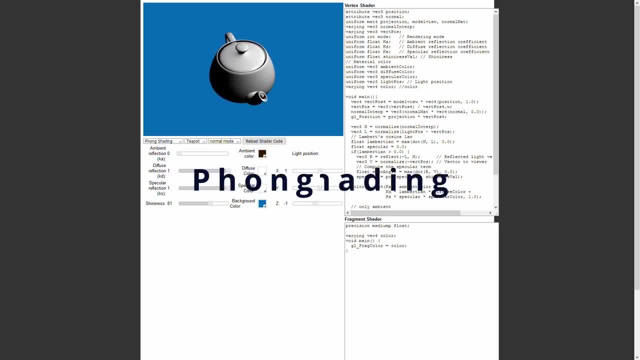 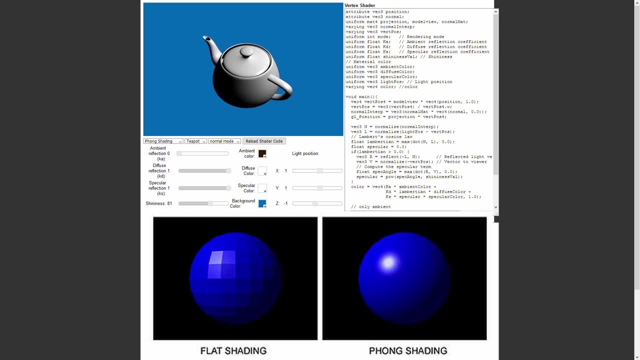 surface looks smooth and much more realistic. This algorithm is called Phong shading and is an example of one of the earliest ways we could render realistic-looking 3d models. But we can do more, because you don't have to stick to realism. Developers can customize their shaders to create all sorts of 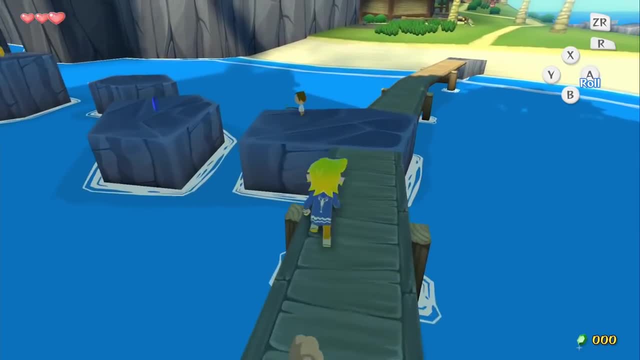 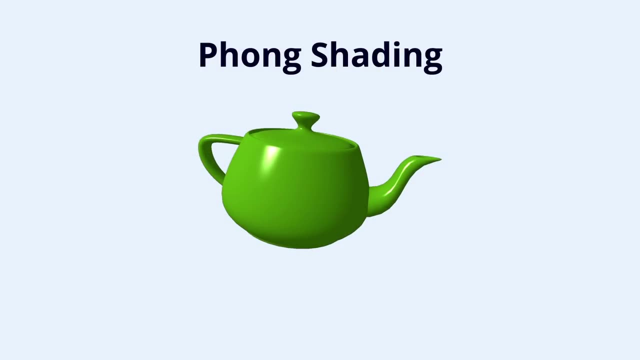 crazy effects. One well-known example which achieves a much more stylized look is cell shading. In cell shading, you start with a regular smooth shading, Such as the Phong shading we just discussed, But now, instead of using a smooth gradient containing all the levels of brightness, we chop up our 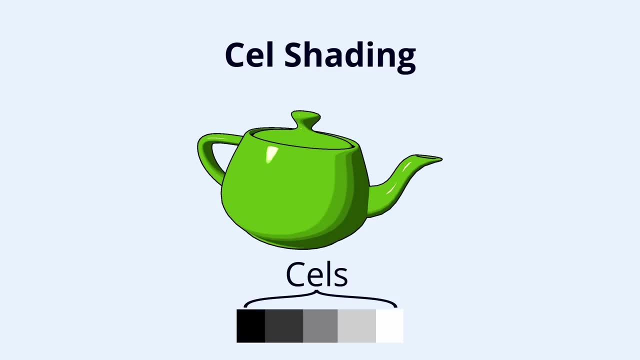 brightness levels into few bands or cells. Only if the brightness level of a pixel falls into another cell does the color of that pixel change, And this way we get a nice cartoony effect. Pretty cool, But so far we only focused on the 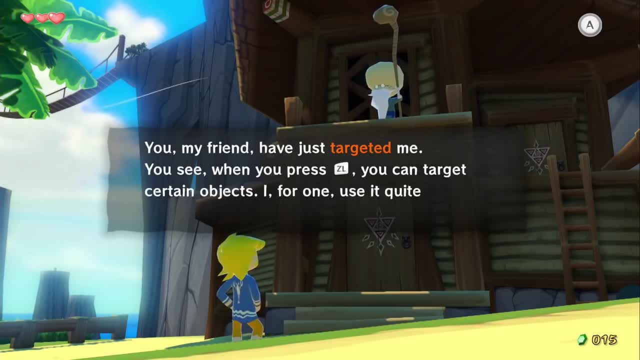 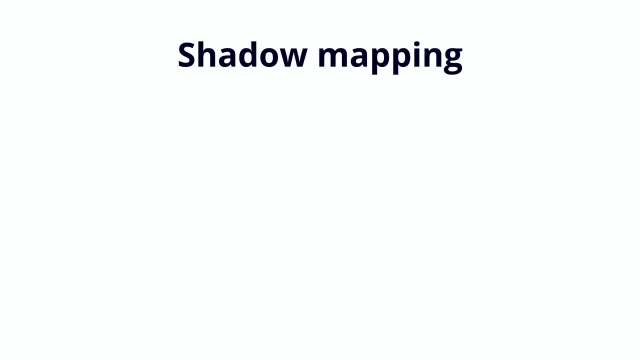 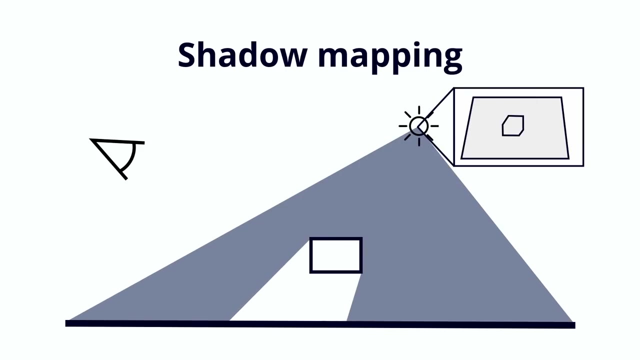 surfaces of objects. We are still missing a very important part to give our scene more depth: Shadows. Shadows and rasterization are generally done using shadow mapping. The way this works is that, essentially, the scene is rendered from the perspective of the light. This gives us a map of which surfaces are seen by the light and 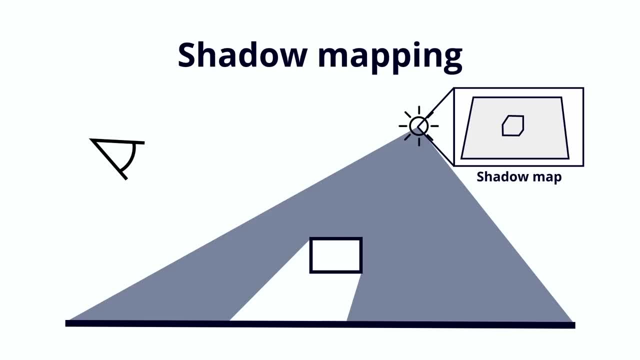 which aren't. This map is called a shadow map. Now, to get the shadows in the scene, we have to find points in the shadow map we just created. If we take this point, for example, we can look up its coordinates in the shadow map. 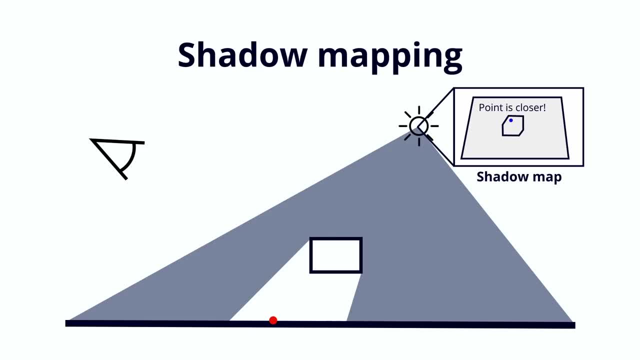 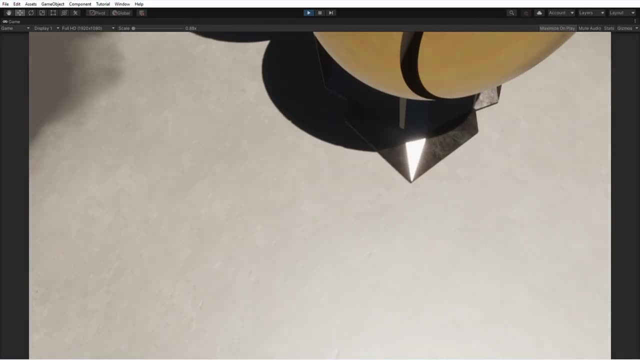 Is there a point that's closer to the light than those same coordinates, Then that means something is blocking the light, which tells us that we must be in the shadows. Of course, this doesn't cover all the techniques involved for rendering shadows. For instance, there are ways to make shadows softer or to take into account different lights. 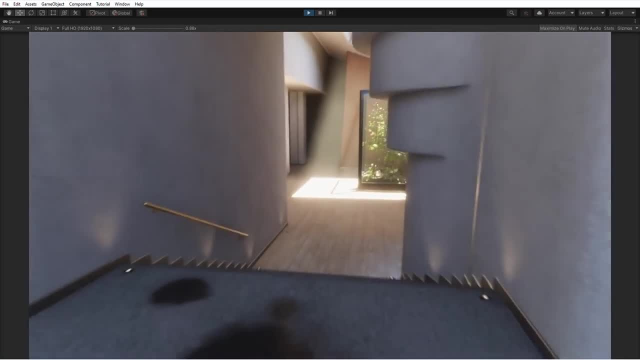 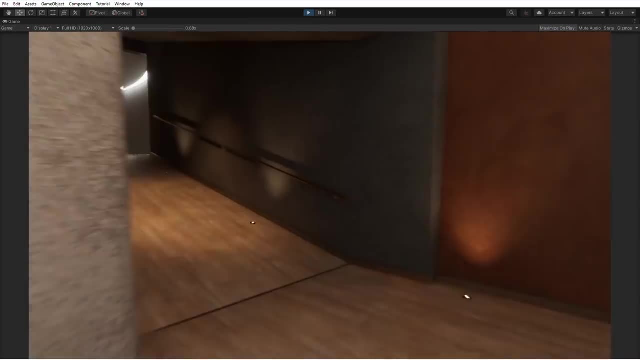 or to account for ambient light bouncing off the environment. There is still much left to discover here, but I just wanted to give you a good sense of how the basics of rendering shadows work in traditional rasterization. Now that we have a lighting setup, things are already looking pretty good. 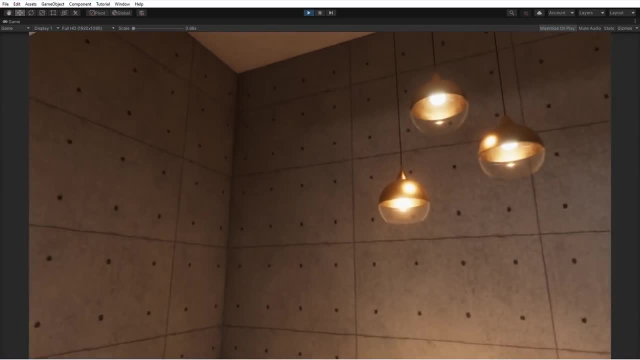 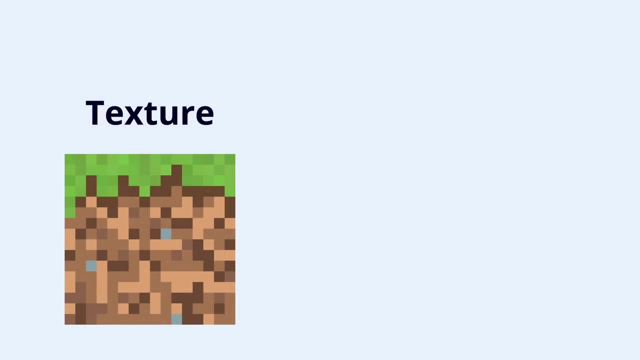 But we still only have flat-colored textureless surfaces. So let's try to apply a texture to our objects. We start with an image we want to use for our texture. Now we need to determine which triangles in our objects will use what part of our texture. 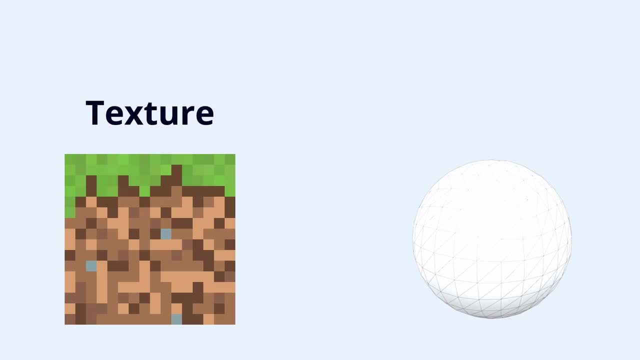 To determine this, we need to generate a UV mapping. You can imagine this as essentially wrapping the texture around our object and remembering where the triangles overlap our image. Now, there are multiple ways to create this UV map, But the principle is the same. 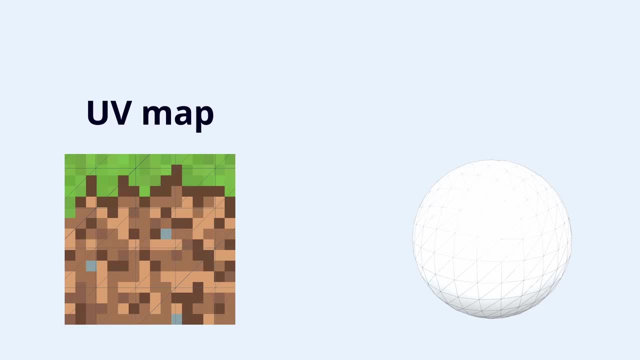 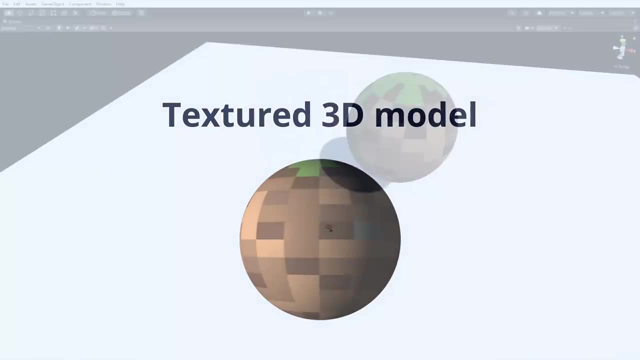 We want to know which triangles should use what part of our texture. Once we have this UV map, we can simply use it to read the colors our triangles should have on our 3D model. So now, instead of a solid color, by using our UV map. 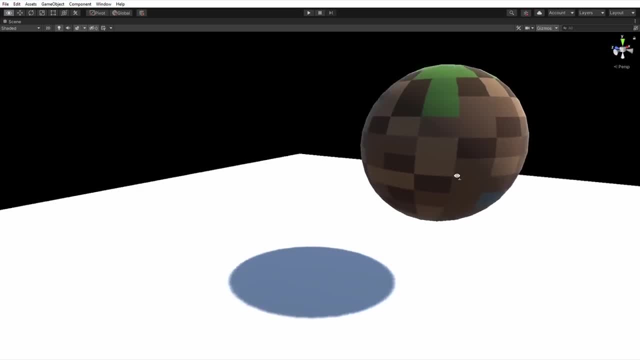 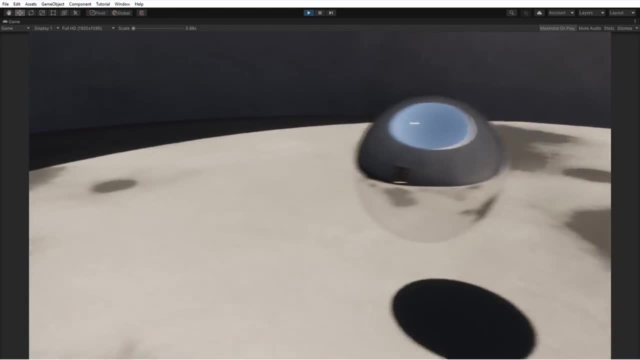 our triangles actually know what part of our texture they should display In rasterization. these UV maps can also be used to fake reflections. In principle, this works by taking a 360-degree picture of the environment and then simply baking it into the texture itself. 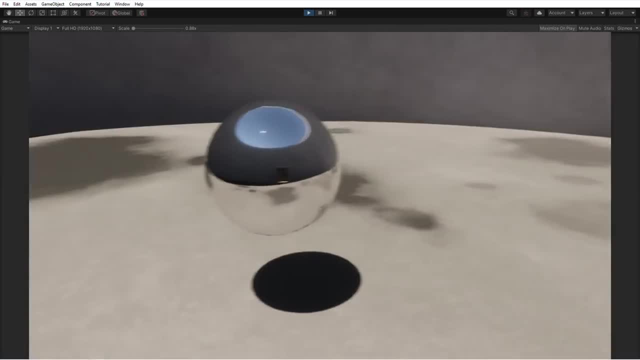 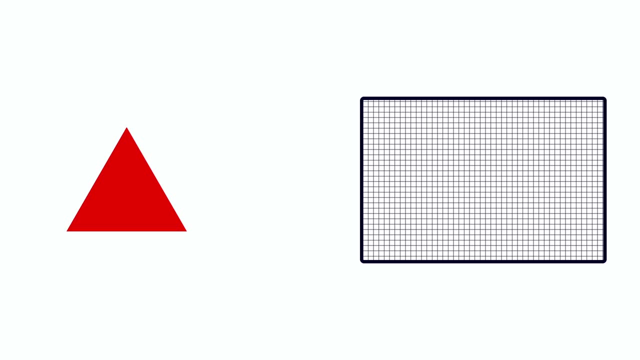 This makes for a very fast and efficient way to show reflections. Finally, we need to display the triangles we created on our screen. Our computer looks at the triangles in our scene and converts those triangles to pixels. However, our graphics card only has so many pixels to work with. 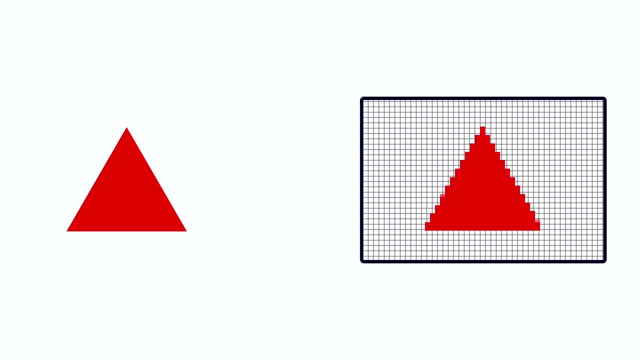 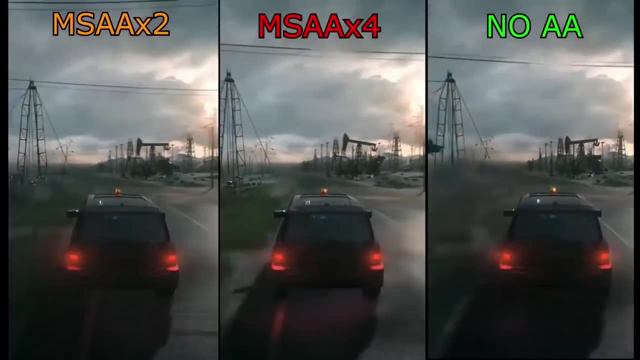 This means that straight lines and edges can become blocky and pixelated. To combat this, graphics cards have to use a technique called anti-aliasing. This adds some extra faded pixels around the straight lines to make them appear more smooth. Once again, there are many different ways of anti-aliasing. 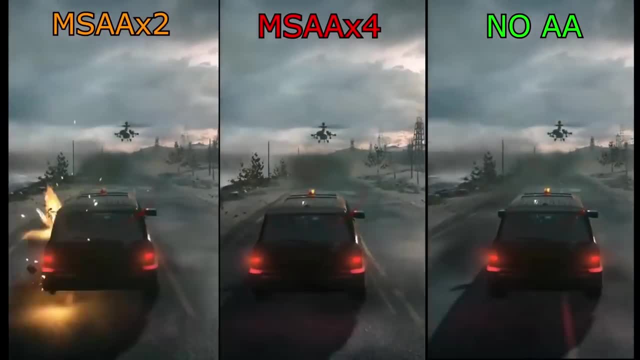 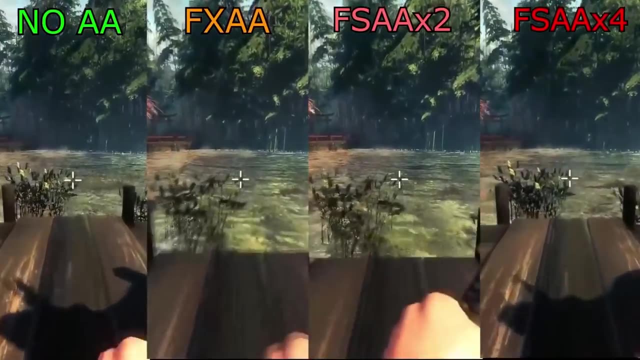 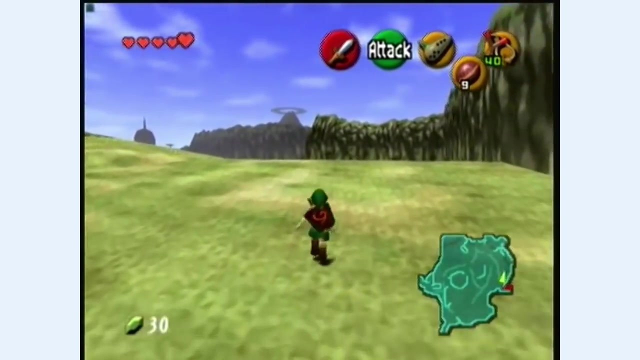 which vary in quality and performance, But they all have the same goal: Make those jagged edges appear smooth. And that covers the basics of rasterization. Of course, these are mostly just simple examples To explain the fundamental principles. In reality, there are much more calculations and shading techniques going on. 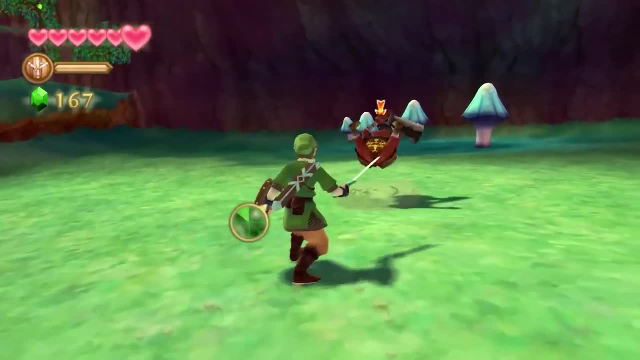 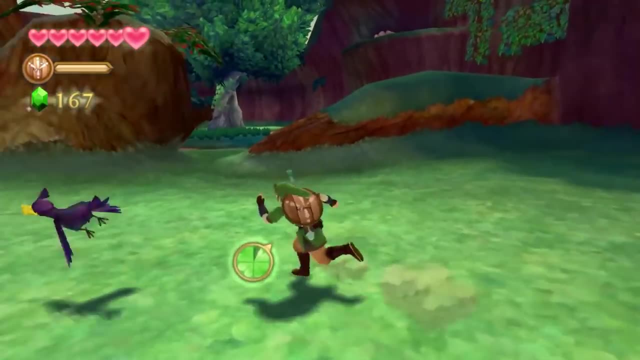 to make objects appear even more realistic. But the basic principle remains the same: Map all the triangles of the 3D models to pixels on the screen and then assign them a color using different shading techniques. This is the basic process that is used pretty much all games today. 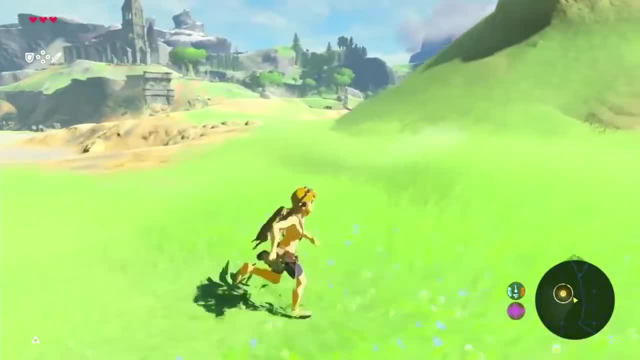 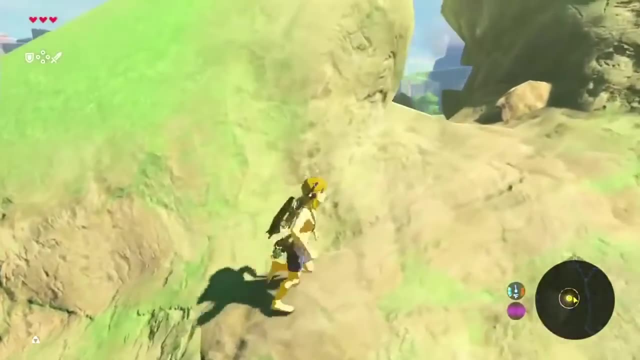 It's fast, it looks good and has proven itself to be a reliable way to render 3D graphics. Over the years, developers have greatly improved and expanded upon these fundamental techniques to achieve the level of realism we see in games today, But there is still much more to explore in the world of 3D graphics. 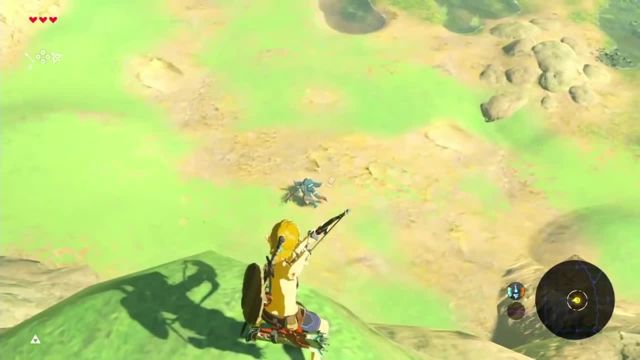 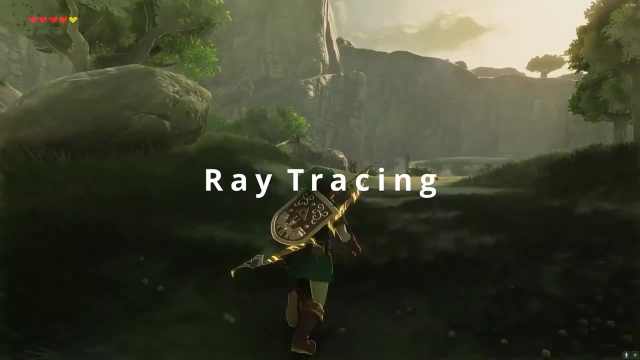 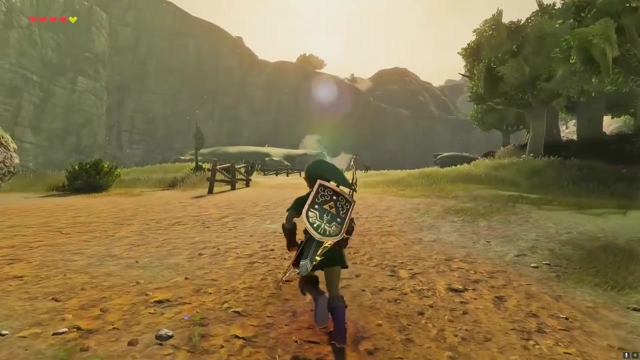 Rasterization is reaching its limits, and game developers are looking more and more towards another technique that can make their games look even more realistic: Ray tracing. But we'll leave that for another video. At least on the subject of rasterization, you're now already a bit wiser.